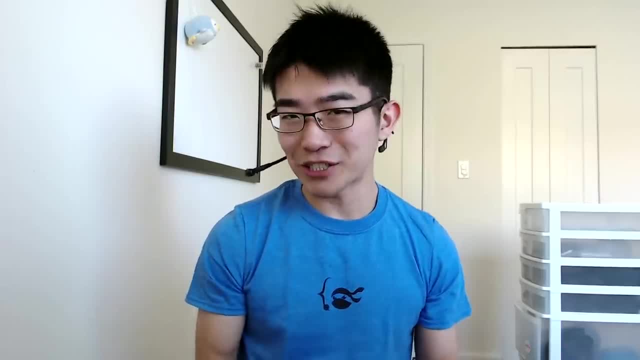 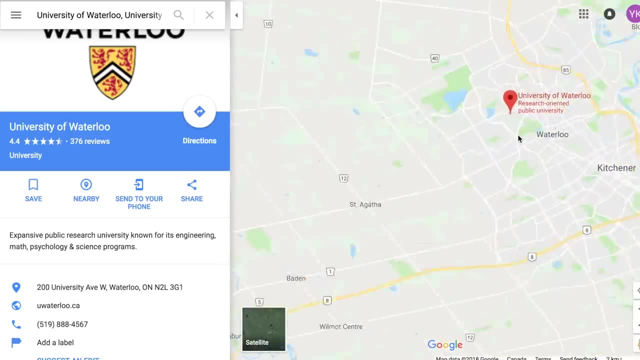 engineer. but let's see what the difference is exactly in more detail, And to do that, I'm going to take a look at the difference between these two majors at one particular university, at the University of Waterloo in Canada, And I chose University of Waterloo for this purpose. 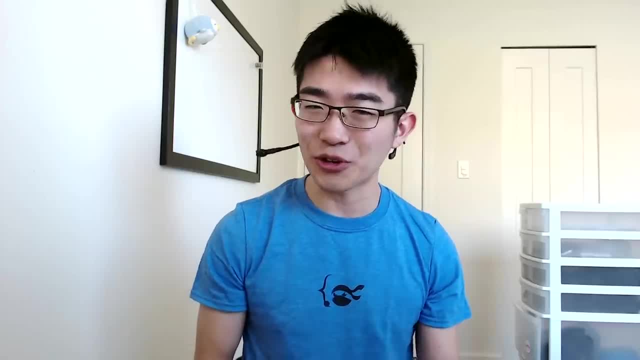 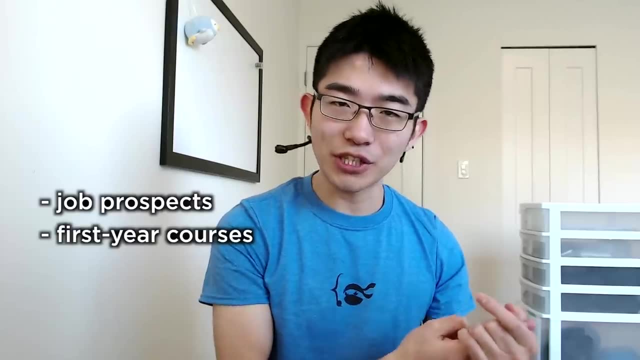 because they have one of the best computer science programs in North America. So I'm going to take a look at a few different things. First of all, job prospects, And then I'm going to take a look at the first year course requirements. 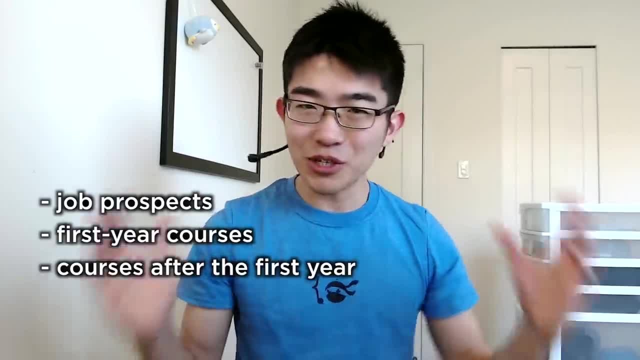 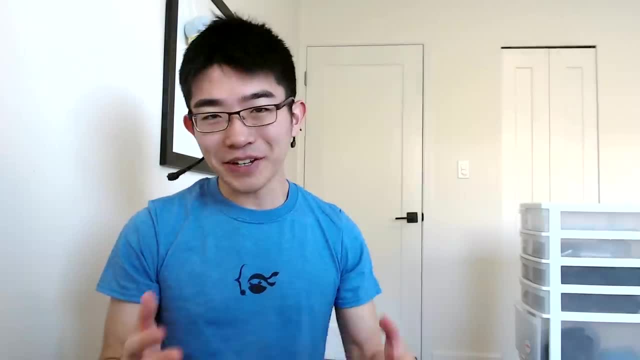 and then the courses required after the first year, And based on all of that, I'm going to draw my own conclusion as to which major is actually better to become a software engineer. Okay, let's first compare the types of jobs and internships you can get through each program. 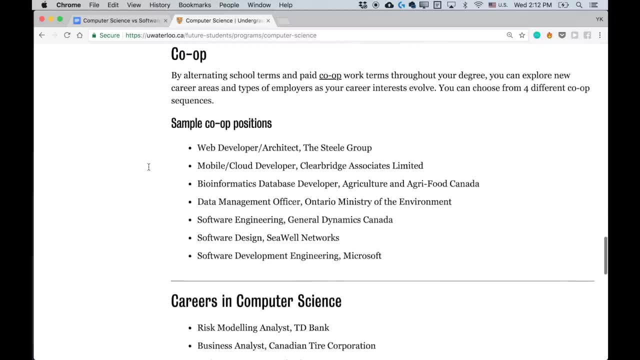 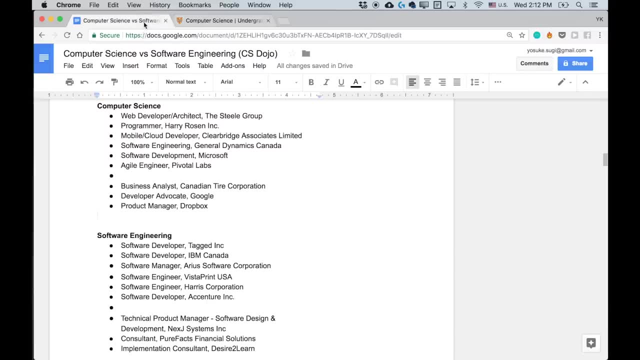 And luckily University of Waterloo's website provides a bunch of examples for this, For co-op or for internships and for full-time positions, And to compare the ones for computer science and software engineering. I pulled a bunch of examples here, And for computer science we have a bunch of. 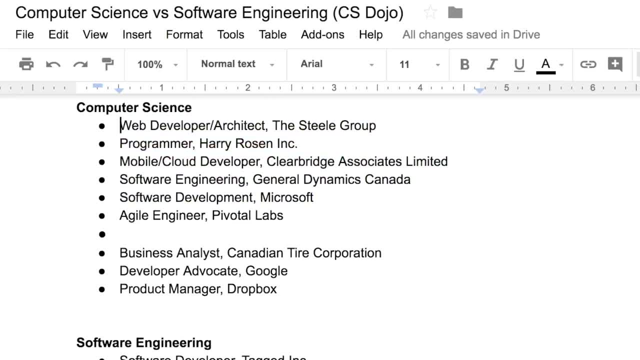 developer and engineer positions, For example, web developer, programmer, mobile and cloud developer, software engineering and so on. They're called by different names, but they're basically all software developer and software engineer, And after that we have business analyst. 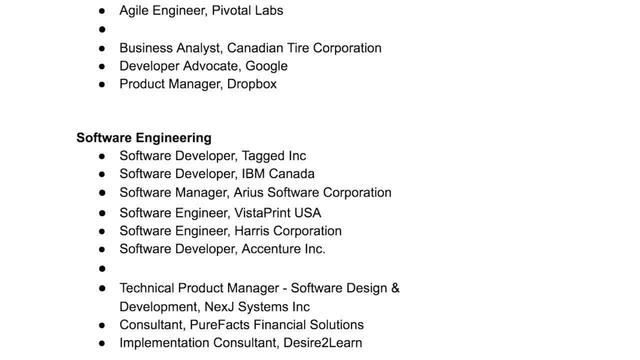 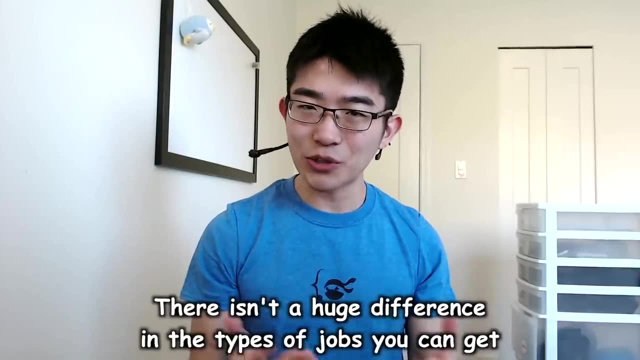 developer, advocate and product manager For software engineering. we also have a bunch of software developer and software engineer positions here, And then technical product manager, consultant and implementation consultant. So what I took away from this list is that there isn't a huge difference between the. 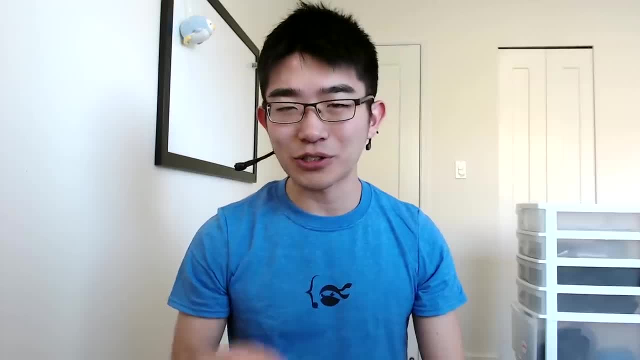 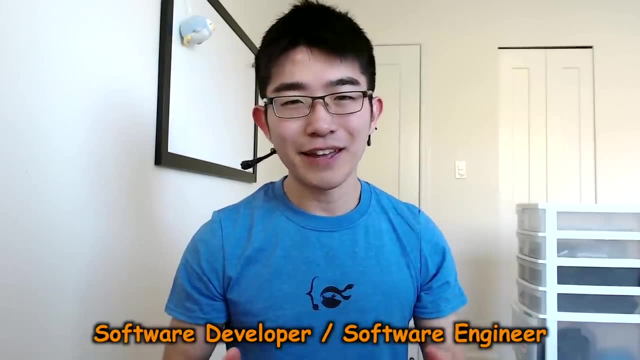 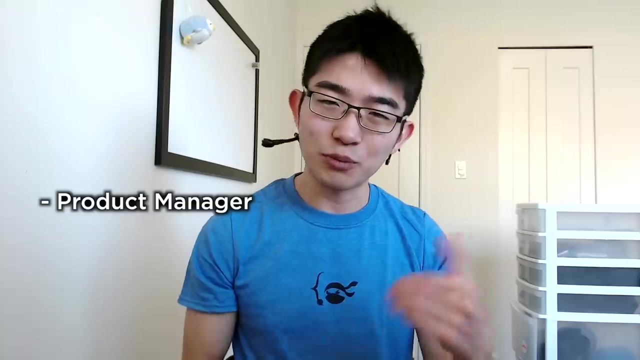 types of jobs you can get through either computer science or software engineering, And the most common job you can get through each program is software developer or software engineer, And these two things are basically the same thing, called by slightly different names. And there are other related options too, for example product manager. 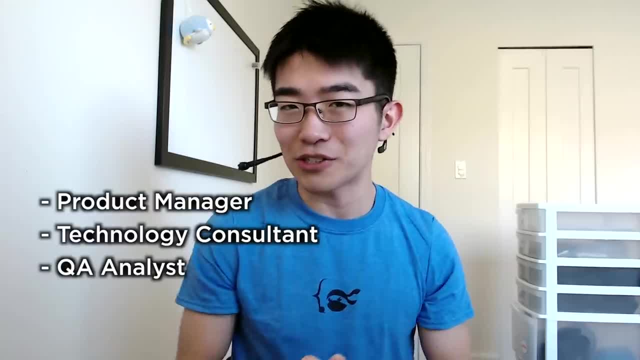 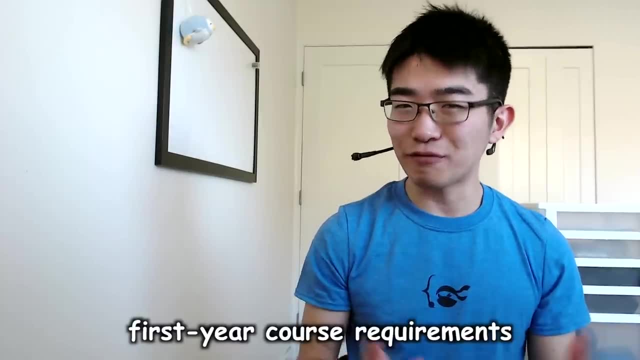 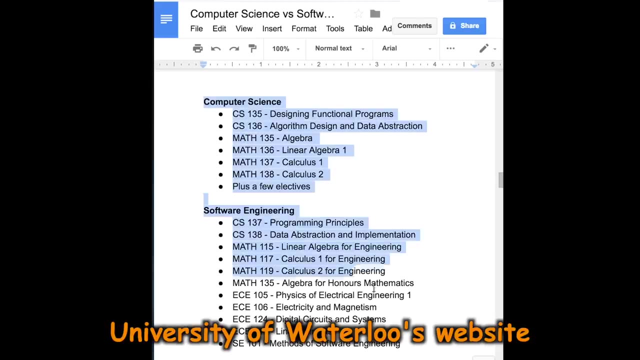 technology consultant and QA analyst, depending on your skill set. Okay, so to get a better idea about what you would actually study in each program, let's take a look at the first year course requirements. So I pulled these requirements from again the University of Waterloo's website, and they're actually pretty similar In computer. 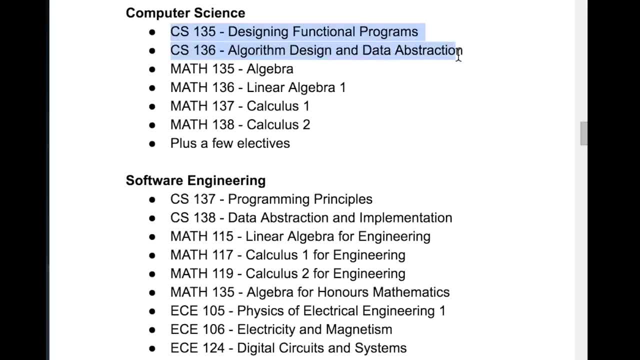 science we have a few computer science fundamental courses And it's same thing in software engineering it's designing functional programs and algorithm design. in computer science And for math requirements we have some linear algebra and calculus courses and that's the same. 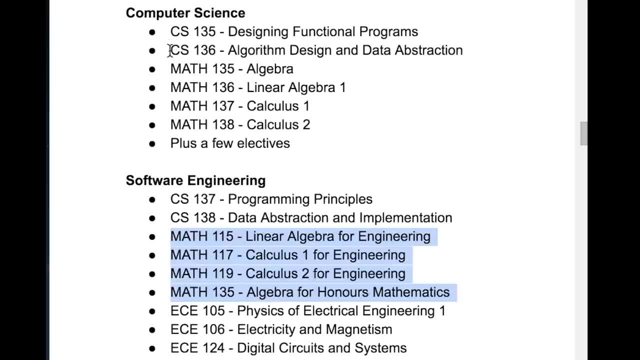 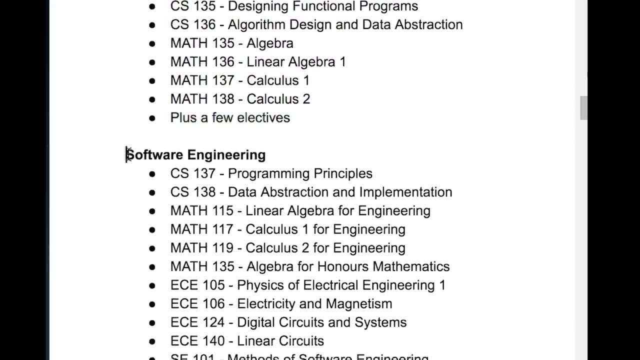 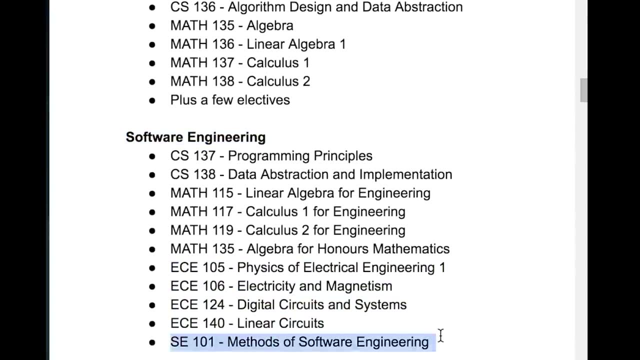 in software engineering. The only difference is that, after these math and computer science requirements, you can take a few electives in computer science, while in software engineering you actually need to take a bunch of electrical engineering required courses and then one software engineering course. Okay, and what about the courses you need to take? 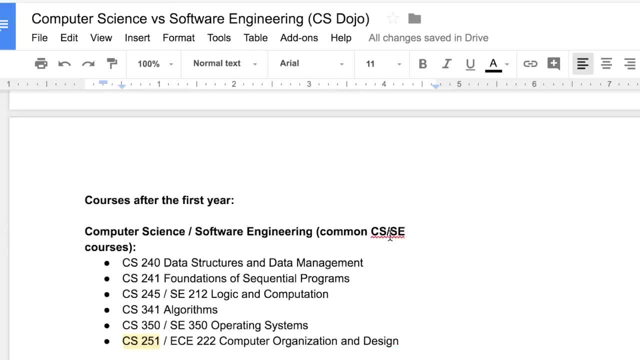 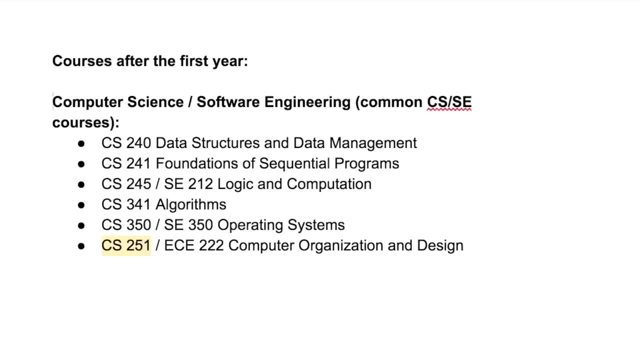 to take after the first year. obviously, after the first year you need to take a lot more courses, so i group them by category so that it's easier to compare. the first category we have here is the common computer science and software engineering courses that you need to take. 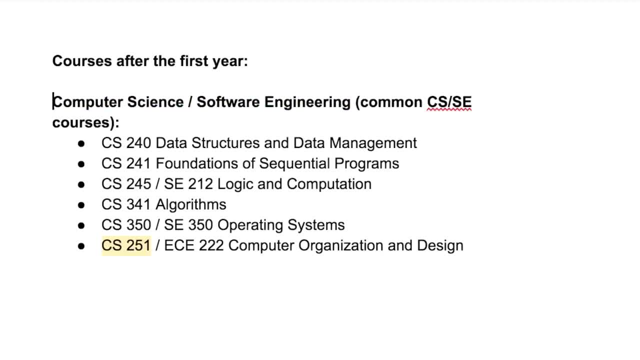 in both computer science and software engineering, and when i saw this list i was actually pretty surprised, because there's a lot of commonality between computer science and software engineering. so we have data structures and data management, foundations of sequential programming, logic and computation algorithms, and then operating systems and computer organization and design and the 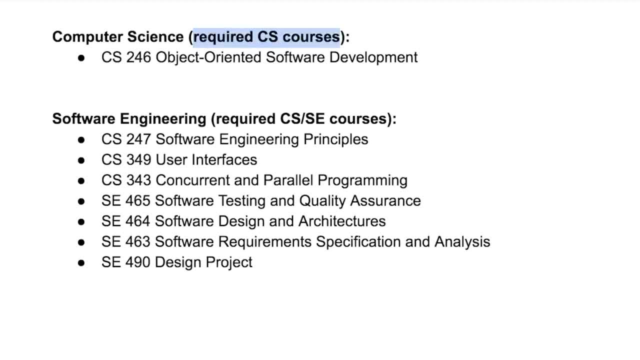 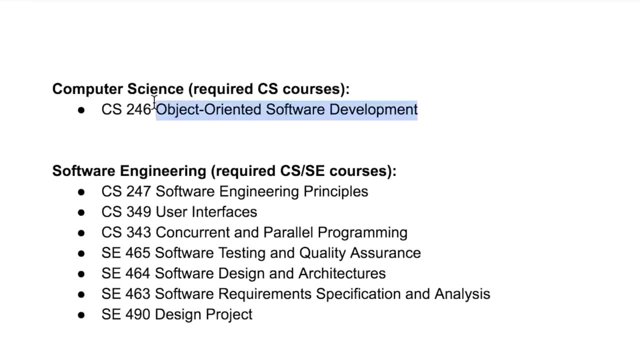 second category i have here is the required computer science or software engineering courses that are required for only one measure but not the other one. for computer science we only have one, which is object-oriented software development, which is actually really important for any type of modern software development and for software engineering. we have a lot. we have software. 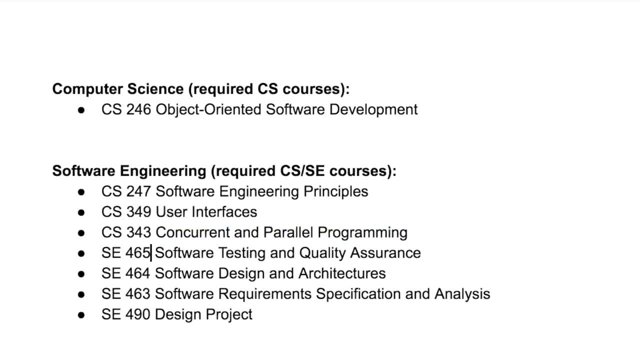 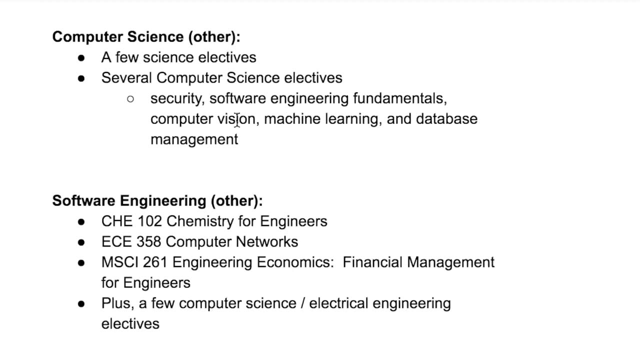 engineering principles, user interfaces, concurrent and parallel programming, software testing, design, requirement specification and analysis and on top of that a design project. so to me it actually seems like a lot of work for software engineering here. okay, let's finish this up by comparing a few more requirements in computer science. you only have a few more science electives and then several more. 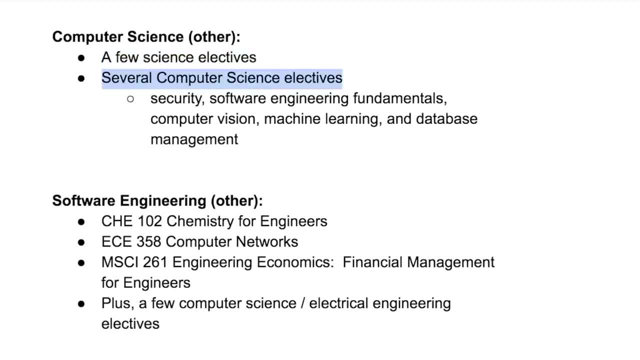 computer science electives. in computer science you only have a few more science electives and then several more computer science electives. you can actually choose them from a wide range of topics, including security, software engineering, fundamentals, computer vision, machine learning and so on, and in software engineering you have a few. 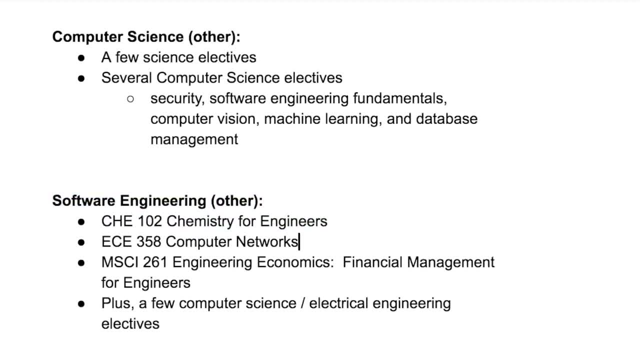 more requirements for engineers. so that's chemistry for engineers, computer networks and then engineering, economics apparently, plus a few more computer science and electrical engineering electives. so i think a consistent pattern that we see here is that there are a lot more requirements in software engineering, while you can take more electives in computer science. so at this point 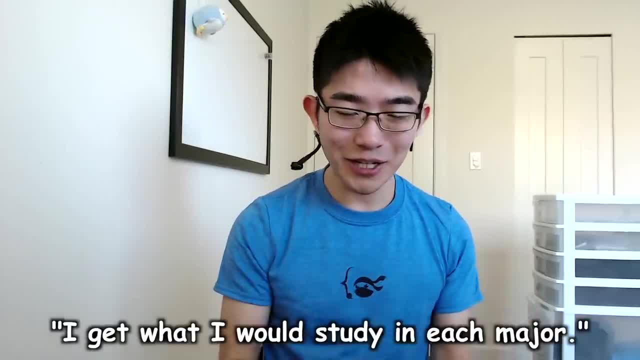 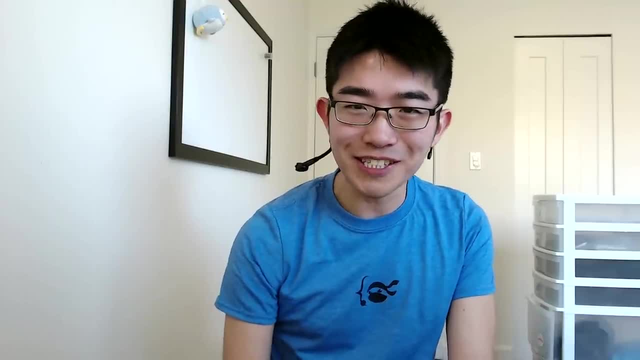 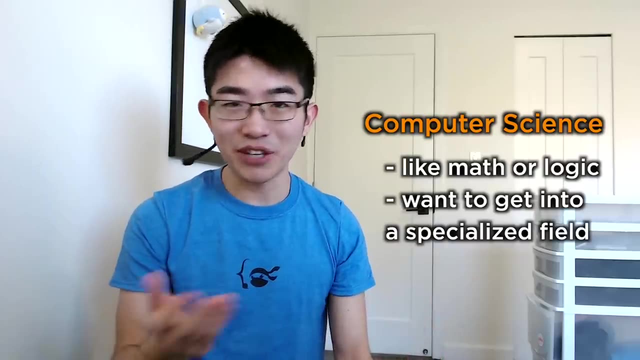 you might say something like: wait, yk, i get what i would study in each major. but which major should i really choose? i think it actually depends on your preferences. so you should choose computer science if you like math or logic, or if you want to get into a specialized field in. 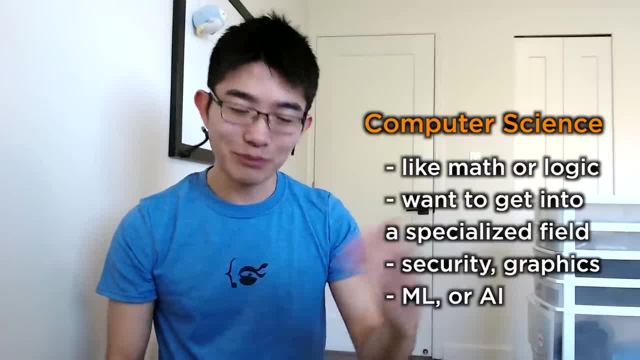 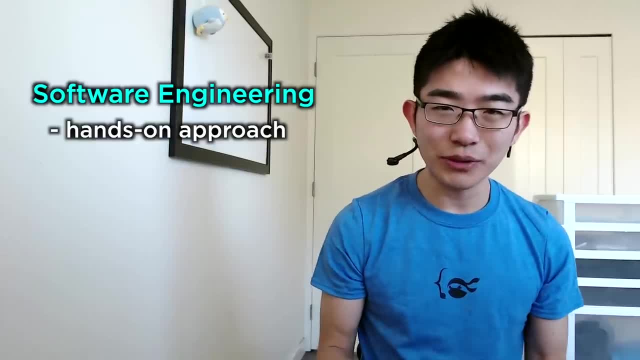 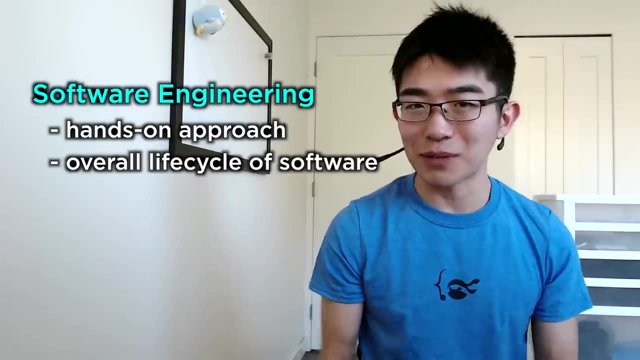 computer science, whether it's security, graphics, machine learning or artificial intelligence, and you should choose software engineering if you're more interested in the hands-on approach or if you're interested in learning the overall life cycle of how software systems are built and maintained. but wait, you might say which one is actually a better measure than to become a software. 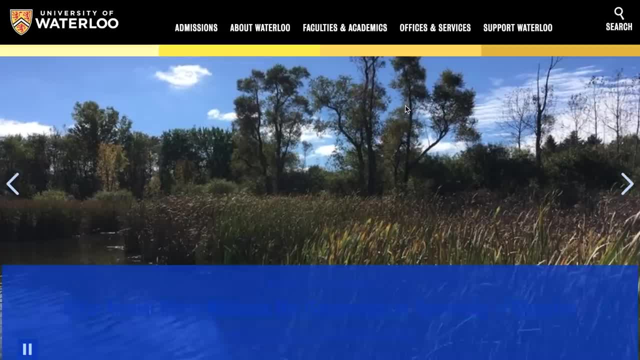 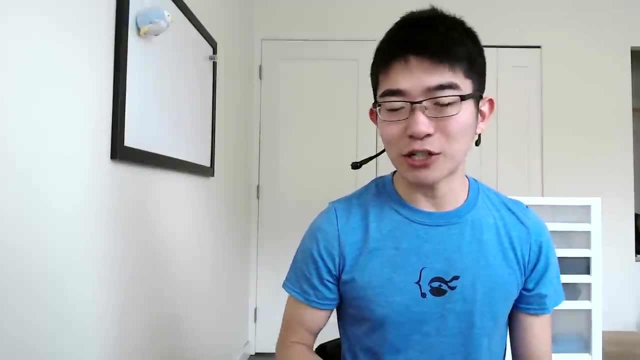 engineer okay. so here's my opinion about that. at this particular university, with this particular set of program requirements, it seems like computer science is a better measure to become a software engineer. to explain why i say that just for simplicity, for now let's just say you're hoping. to get one of the highest paying jobs as a software engineer in north america, and these jobs typically pay, you know, about a hundred thousand dollars or even more, and these jobs are typically at a large software company, for example microsoft, amazon or google, or at a medium-sized high growth. 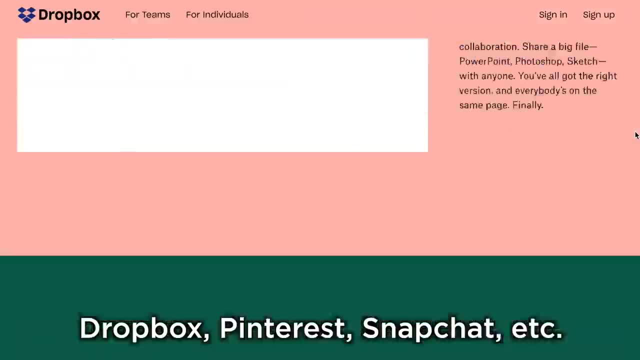 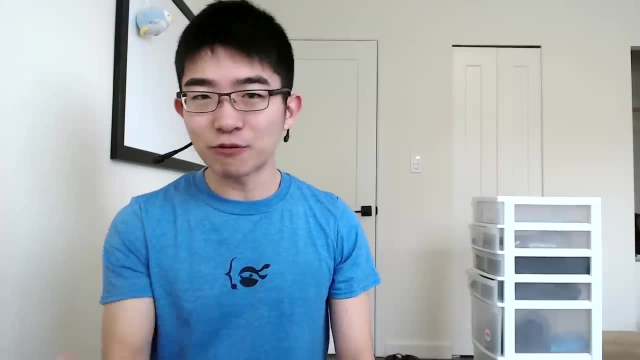 so think dropbox, pinterest, snapchat and so on, and of course not everyone wants to get this kind of job. but let's just say, for simplicity, for now that's, you know, at least one of your options. so typically, what these companies look for in a software engineer candidate is the ability to 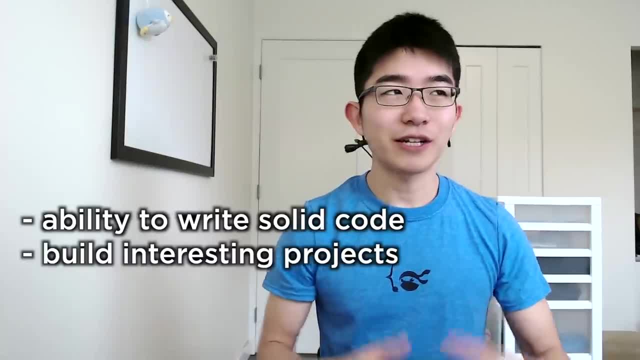 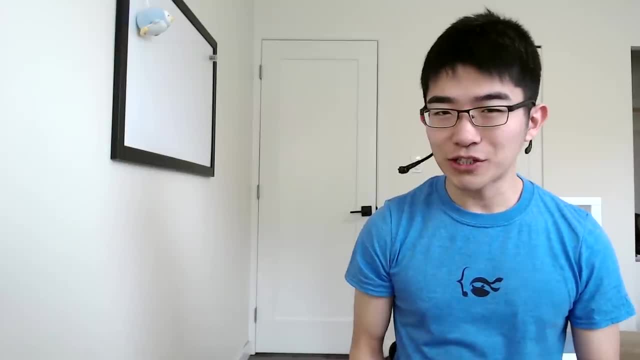 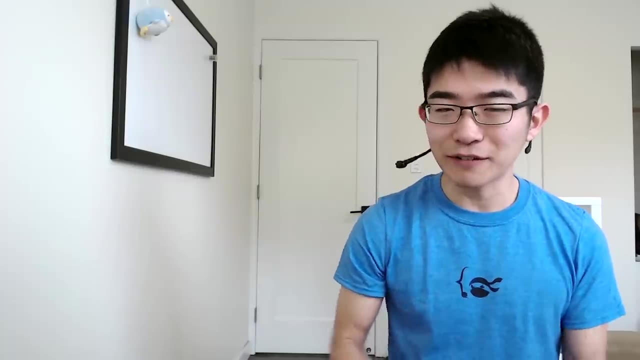 write solid code and build interesting projects, as well as you know your computer science fundamentals, including data structures and algorithms, and i think the best way to cultivate these skills is by quickly learning computer science fundamentals and then spending your own time after that practicing solving problems, writing code and building interesting projects and, i think, based on the 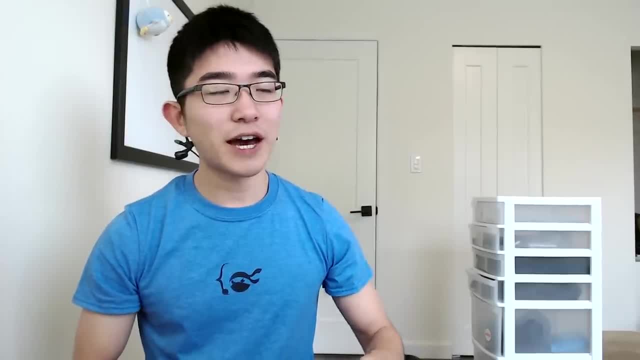 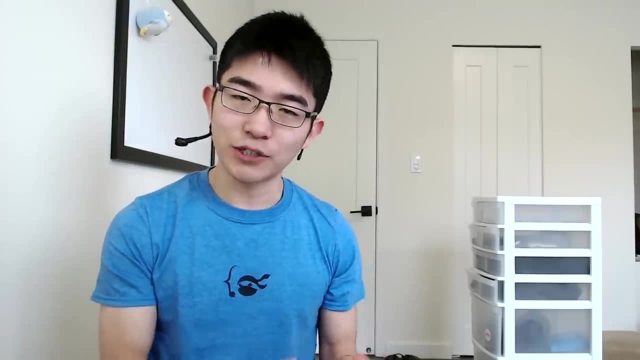 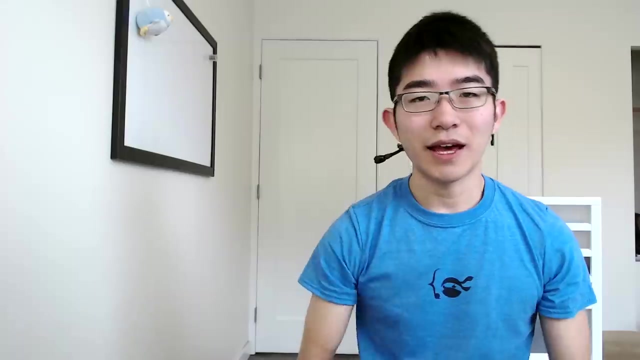 curriculum for software engineering and based on how busy you know engineering students tend to be in general, i think it would be much, much harder to do that with software engineering than with computer science, because with software engineering you'd be just so much busier with the required courses and 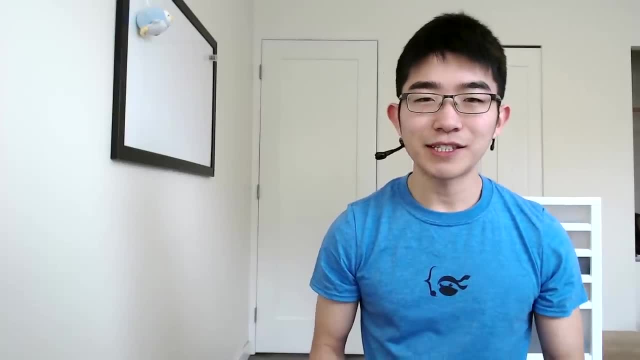 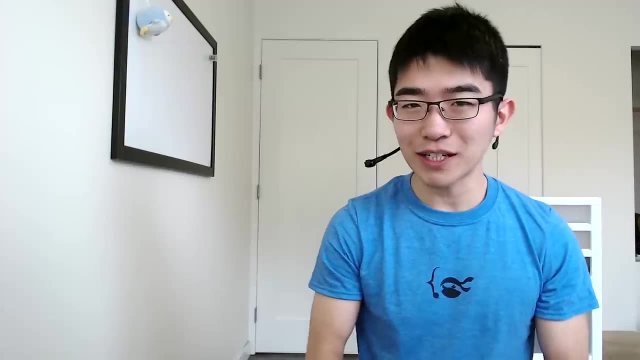 another benefit of this particular computer science program is that it allows much more computer science electives. and that's great because based on what's in demand in the job market you know right at the time you graduate. you can adjust your courses. so, for example, if mobile app 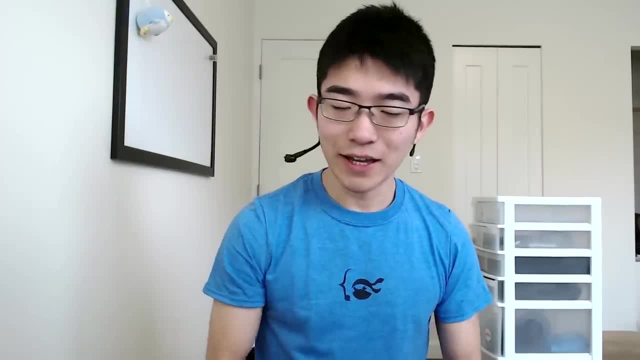 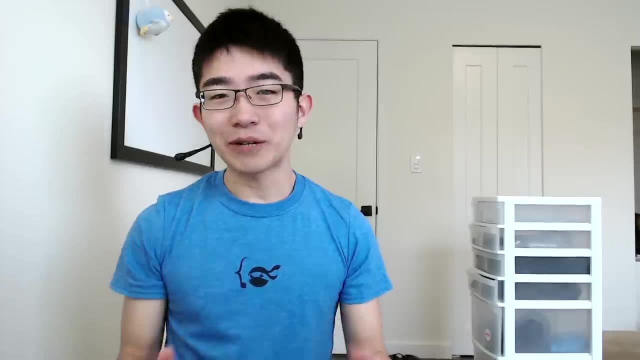 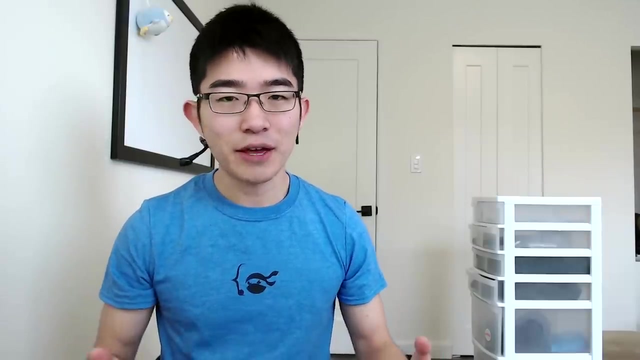 development is in demand right now, you can learn that, and if machine learning happens to be in demand in a job market right now, then you can focus on that instead. so i'm sure there are some benefits to learning software engineering fundamentals, for example, software testing and design and so on. but 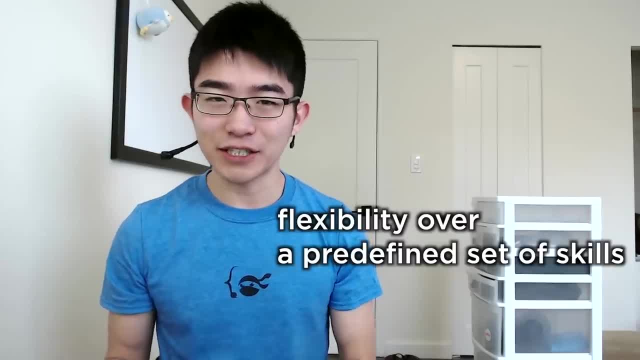 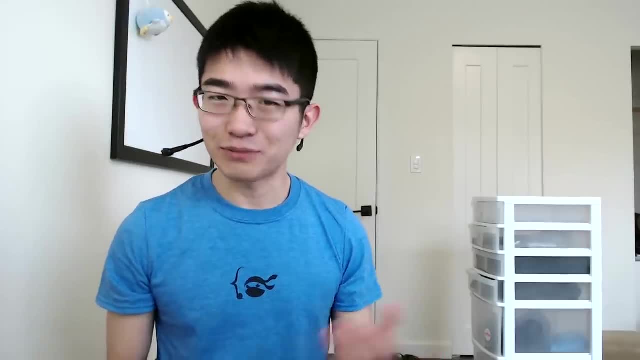 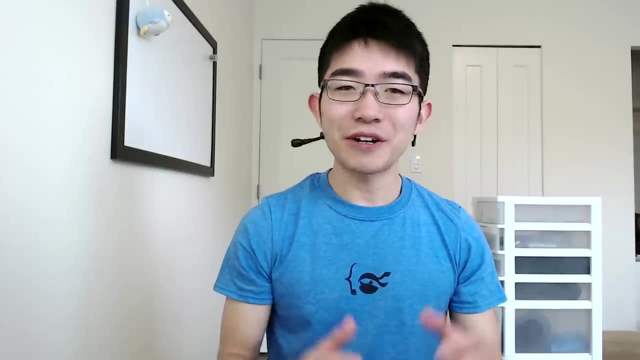 i would personally rather take flexibility over a predefined set of skills, and that's why i think computer science is a better measure to become a software engineer with this particular set of program requirements at least. okay, once again, that's just my opinion, based on one particular university, so there are a few more things to keep in mind. first of all, obviously different. 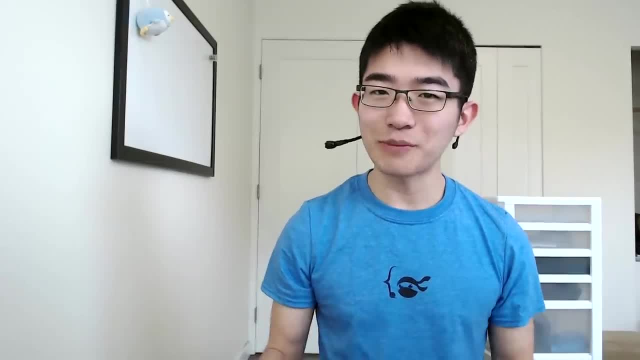 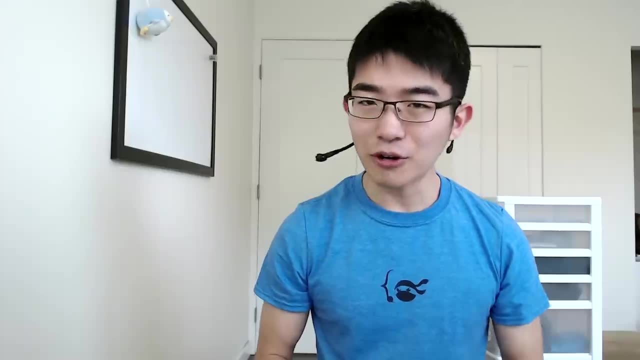 universities have different program requirements for computer science and software engineering. so this video should be a good starting point, but before you decide, you should definitely take a look at the program requirements at the particular university you're interested in attending. and the second thing to keep in mind is that some universities don't even have a software engineering. 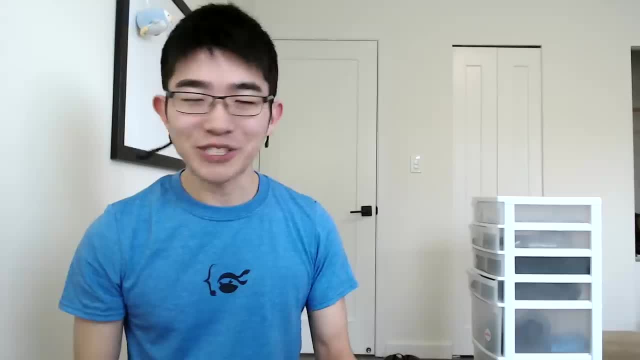 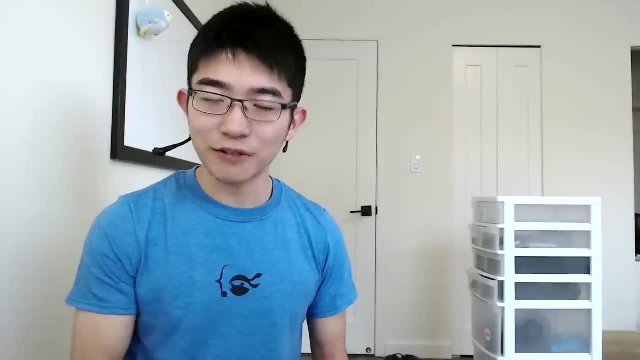 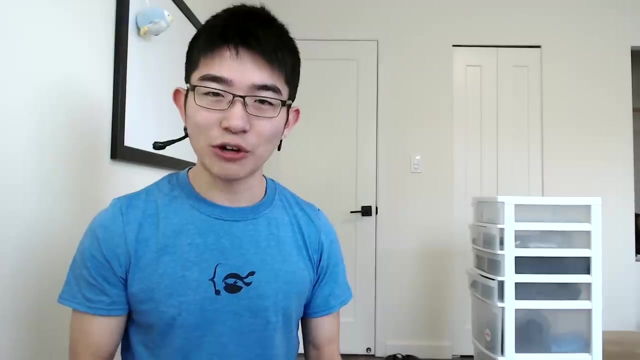 major. for example, the university i went to, the university of british columbia in vancouver. it doesn't have a software engineering major, even though it has computer science and computer engineering. so if you're interested in computer science you can go to the university of british columbia if the university you want to go to doesn't have a software engineering major. 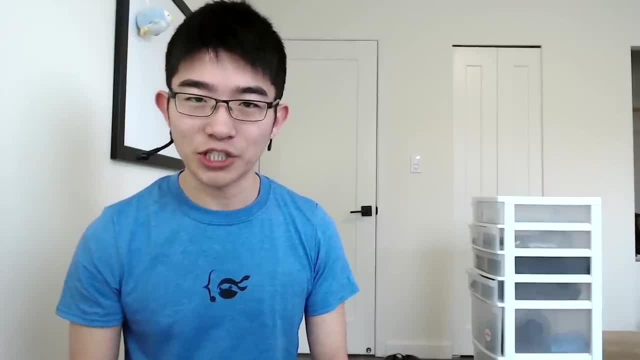 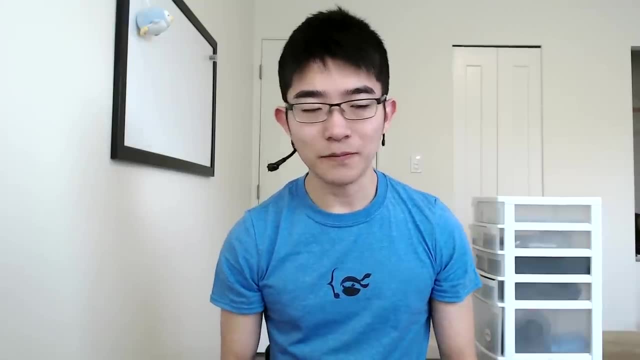 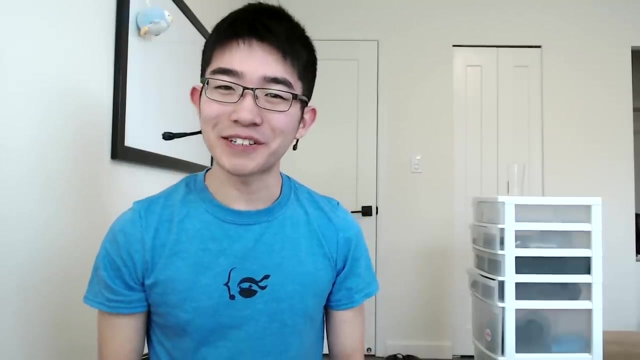 i would just go with computer science if you want to become a software engineer. so computer engineering is more focused on hardware than software engineering or computer science major, so it's less directly related to a typical software developer's job. okay, i'm kind of curious: what's your opinion on this? do you agree with me or disagree with me?